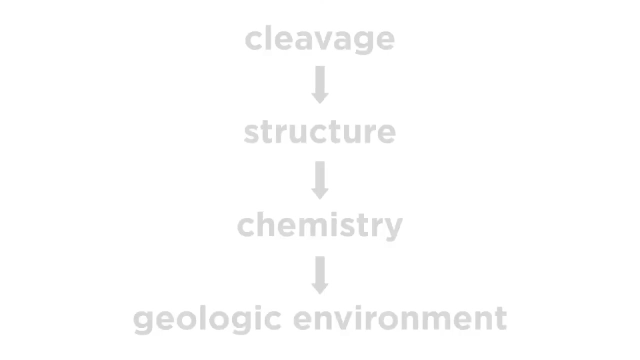 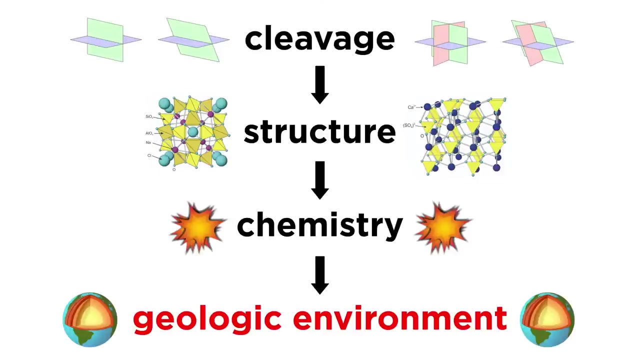 in atomic radii and bond lengths. This means that from a clear, macroscopic property like a mineral's cleavage, we can potentially know something about its structure, which we can relate to its chemistry and which we can use to know something about the geologic environment in which it formed. Of course, this does not always. 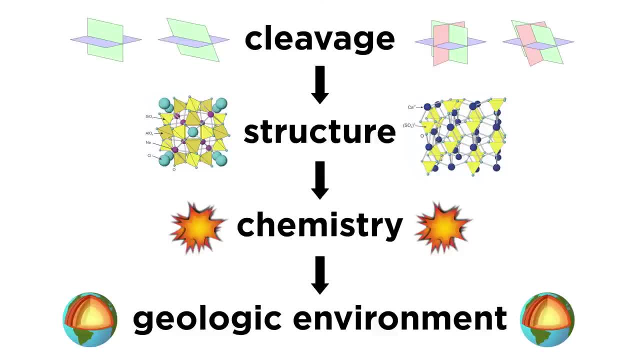 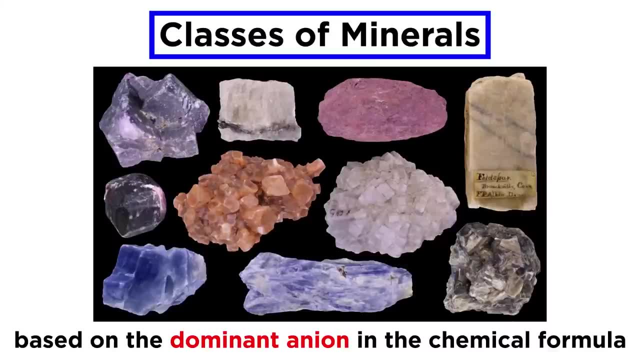 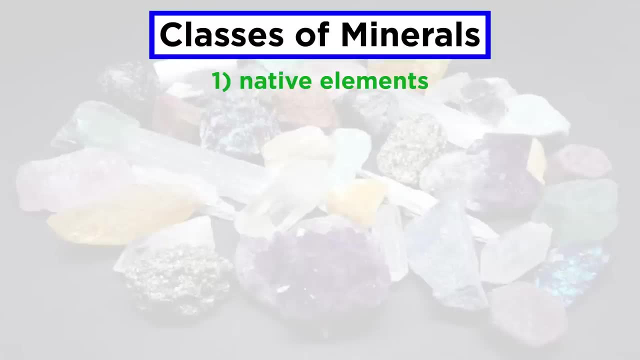 work. However, it is a simple logical framework that geologists use to determine a rock's history. Minerals are divided into eight classes, based primarily on the dominant anion in their chemical formula. The eight classes are as follows: Native elements, oxides. 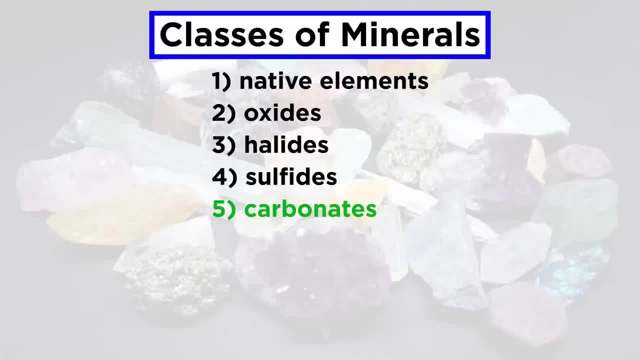 halides, sulfides, carbonates, sulfates, phosphates and silicates. Moreover, an additional class mineraloids is reserved for geologic materials that lack a crystal structure and therefore are not minerals. Many of these terms should already be familiar from our study. 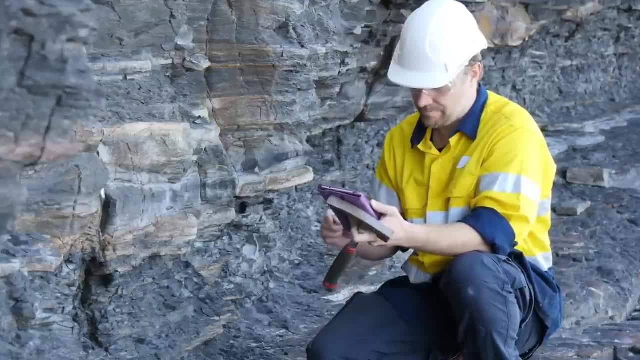 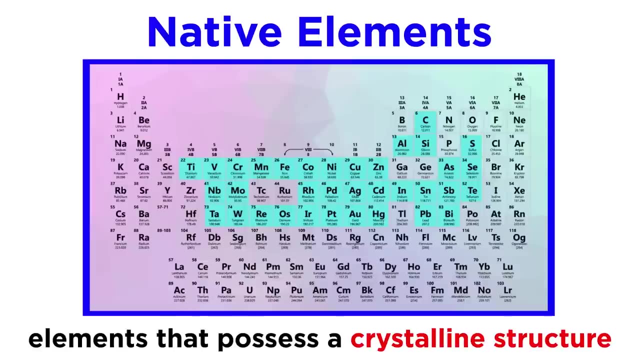 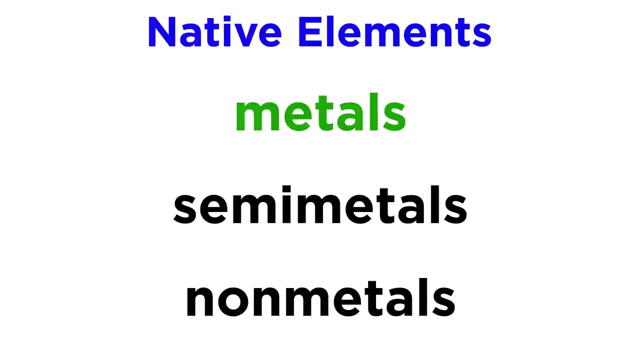 of chemistry, but either way, let's make sure we contextualize them in our study of geology. Let's begin with the simplest class of minerals: Native elements. As the name suggests, they are naturally occurring elements that have a crystalline structure. They are divided into metals, semi-metals and non-metals. 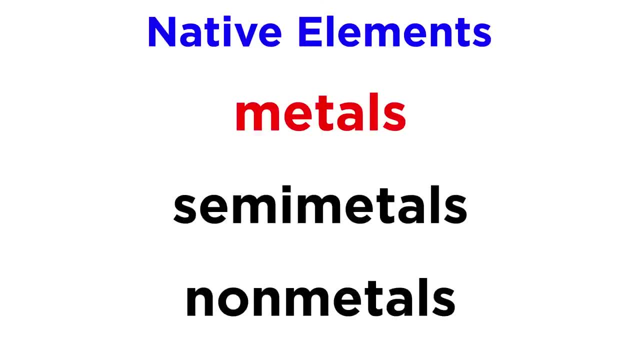 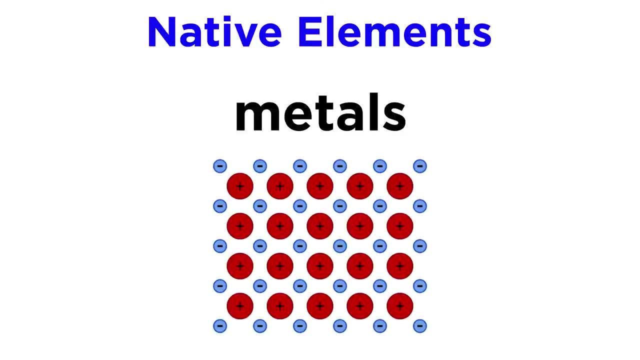 Native metals will be of the greatest interest to us, as they form most of the native elements. Remember that what makes a metal a metal is the propensity to have delocalized valence electrons that are shared among all its atoms. Most native elements are relatively 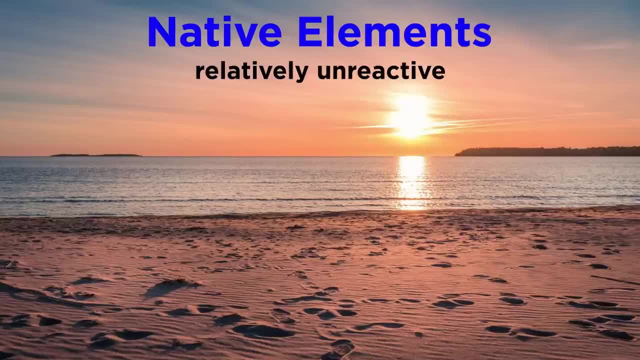 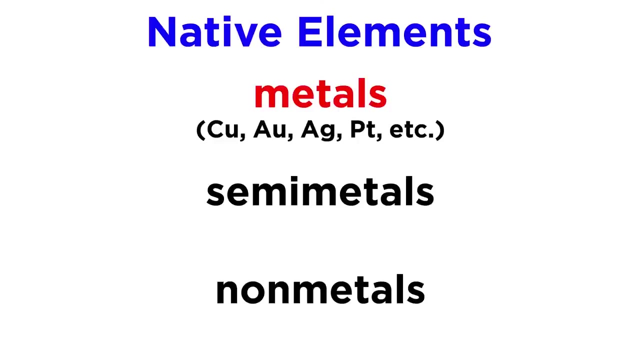 unreactive, Which is evidenced by their existence in such oxidizing environments as Earth's surface, where oxygen and water are readily available to form oxides and hydroxides. Some examples of native metals are copper, gold, silver and platinum. The native semi-metals are: 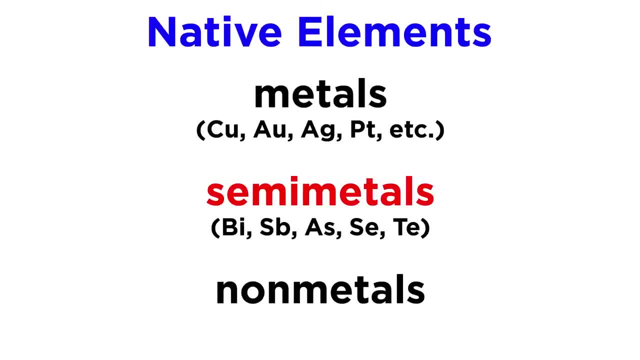 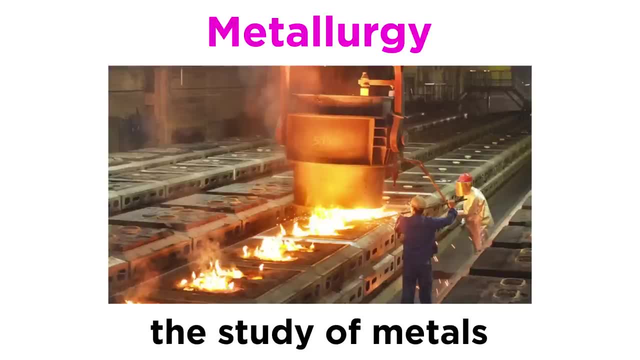 bismuth, antimony, arsenic, selenium and tellurium, And the only two native non-metals are sulfur and carbon. Here's an entire field of science called metallurgy that is completely based on the study of metals. You can imagine the importance of metallurgy in the modern age when considering 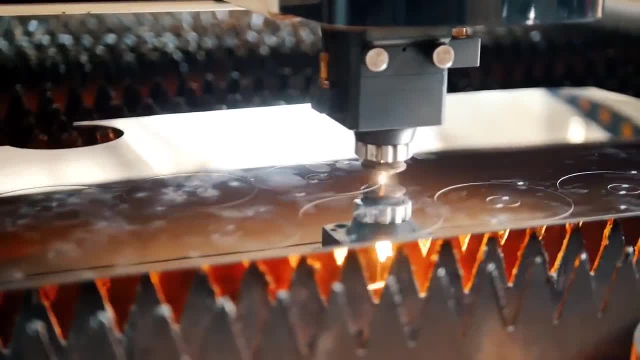 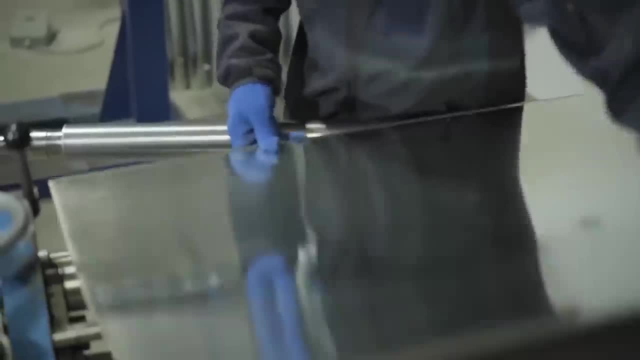 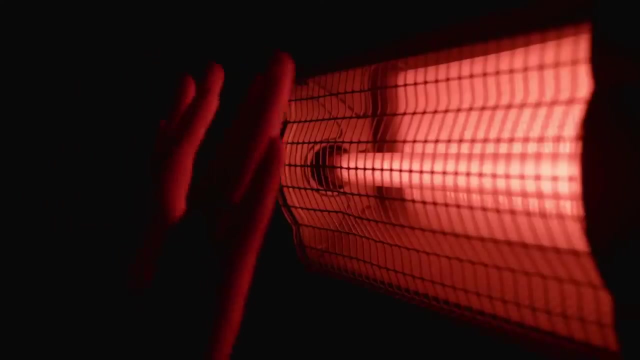 all of the different properties of metals that are required for specific applications, such as electrical conductivity, superconductivity, rigidity, flexibility, mag華tism and high melting point. For example, electric heated elements required an alloy that is ducted to air. Claus, derived from a material-스터ic type of silvery sheet, where the sensor reacts by falling, weren't particularly charged to a rocket effect influx, dancing off the experiment by adding brilliant results displayed showing that it will accept black light at or. Brain is one of the chemical temperature sources of smoke. 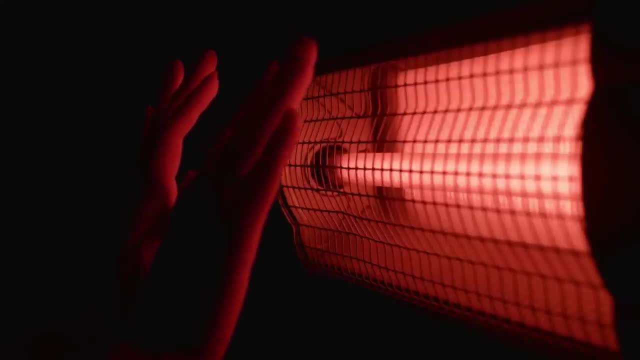 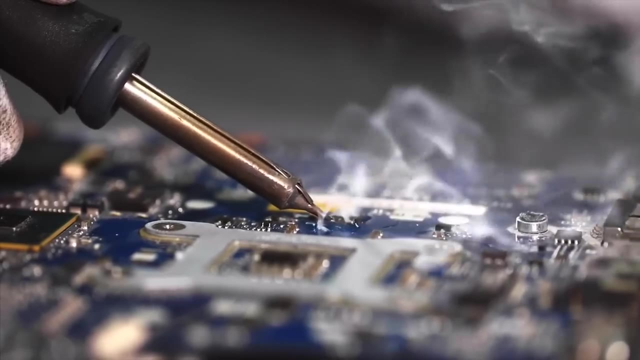 volatile, with a high electrical resistance and melting point, whereas solder, which is used to connect wires to circuit boards, must have a low melting point and low resistivity. Furthermore, you wouldn't even be able to watch this video without the single crystal. 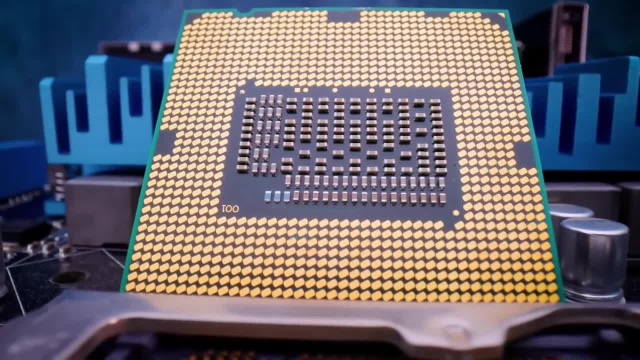 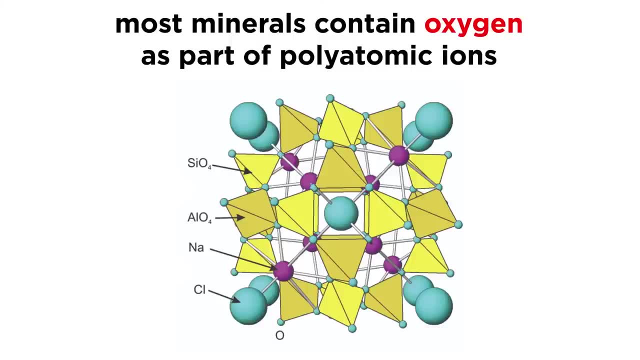 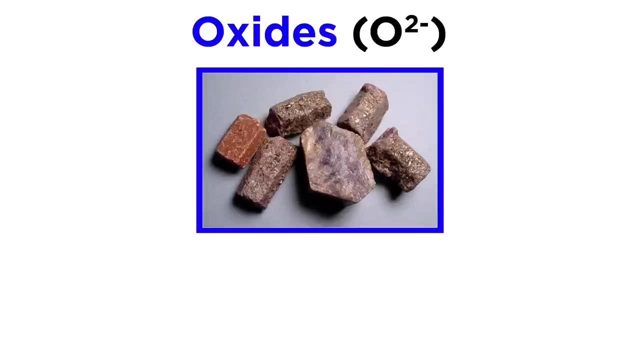 silicon in your computer's central processing unit. Thus the incredible importance of understanding minerals. Since most minerals contain oxygen, such as with silicates and carbonates, the oxide class is restricted to minerals where one or more type of cation is ionically bonded, only to 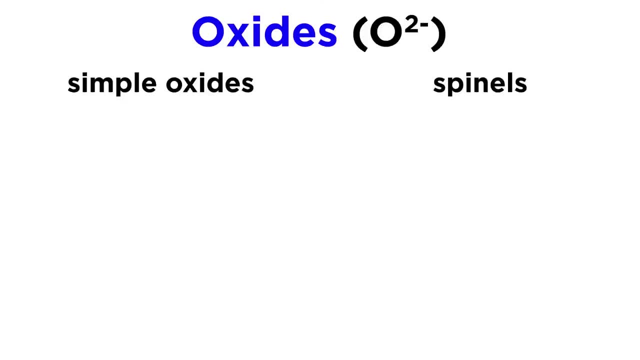 oxygen Oxide minerals can be broken down into two groups: simple oxides, which only contain cations of identical charge, and the spinels, which contain cations of dissimilar charge. The simple oxides can be further grouped based on the charge. 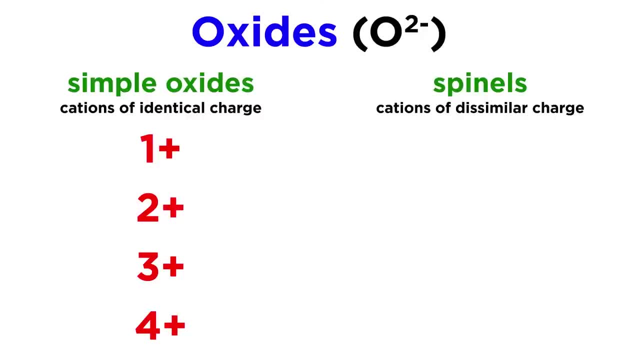 of their cation, which is usually between one and four. Some examples of simple oxide minerals are cuprite, a monovalent copper oxide, periclase, a divalent magnesium oxide, hematite, a trivalent iron oxide, and rutile, a tetravalent titanium. 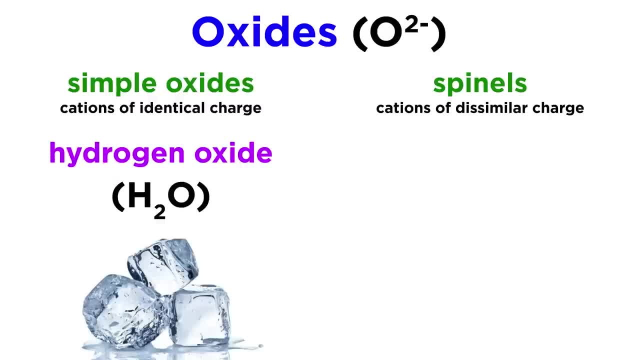 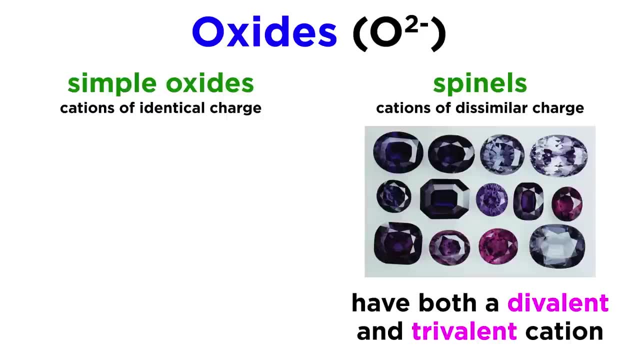 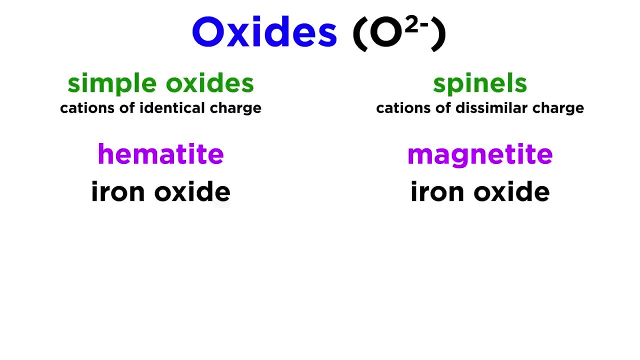 oxide. Another instantly recognizable monovalent oxide mineral is hydrogen oxide, which is more commonly known as hydrogen oxide. The spinels are a bit more complicated, having both a divalent and trivalent cation in their chemical formula. Magnetite is an iron oxide like hematite, but it contains both ferric and ferrous iron. 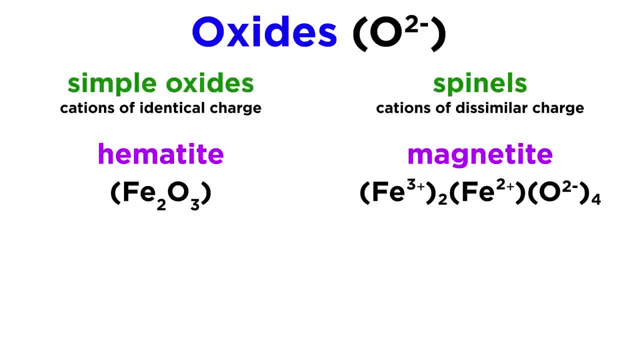 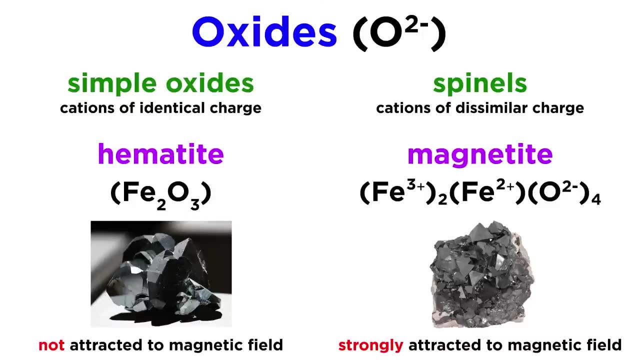 having a chemical formula of Fe3 plus 2, Fe2 plus O2 minus 4.. The difference between magnetite and hematite is clearly highlighted by their magnetic properties, as magnetite is strongly attracted to a magnetic field, whereas hematite is not. 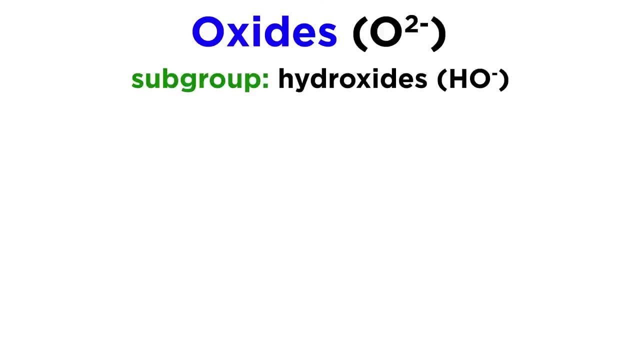 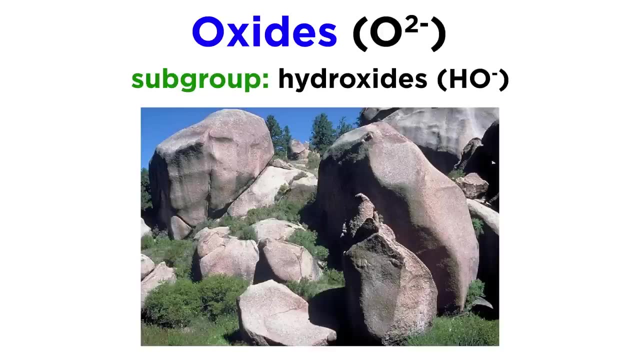 An important subgroup of the oxides is the hydroxides, which are composed of cations that are bonded to a hydroxide ion. They are commonly produced by chemical weathering or alteration of other minerals as they react with precipitation and groundwater near the surface. 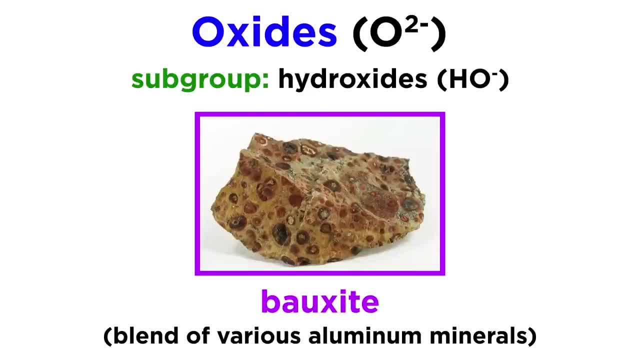 Bauxite, which is the dominant ore of aluminum, is composed of several aluminum oxides which are also the dominant ore of aluminum. Bauxite, which is the dominant ore of aluminum, is composed of several aluminum oxides and. 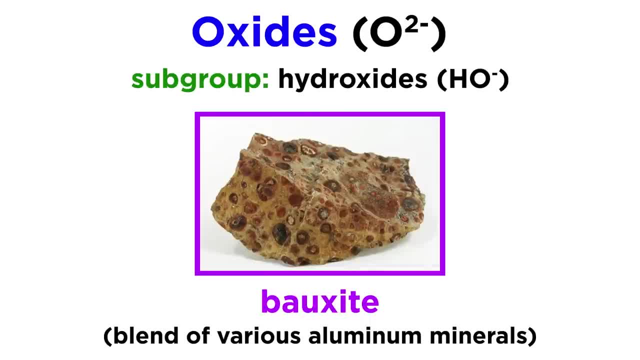 as you can see in the video, is composed of several aluminum oxyhydroxide minerals that form in tropical environments where abundant precipitation and high temperatures intensely leach everything out of the rocks except for aluminum, which is one of the most immobile. 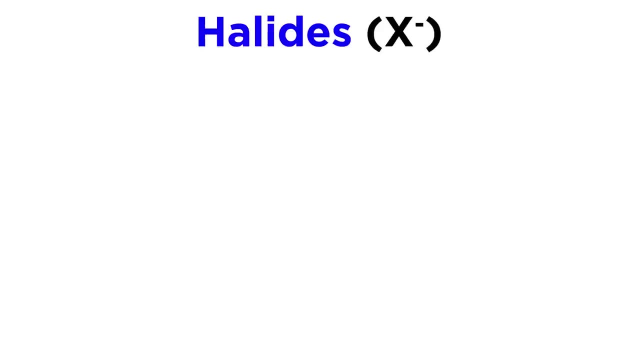 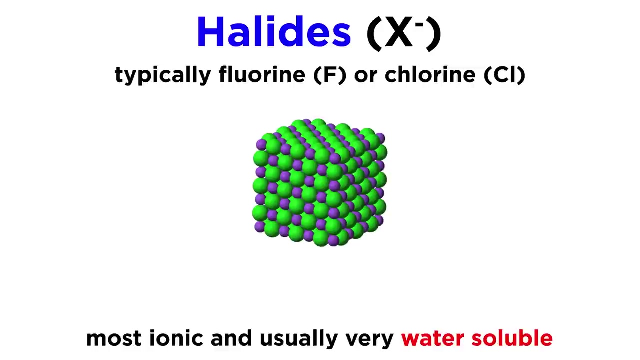 and insoluble geologic materials. Another simple class of minerals with ionic bonding is the halides, which are composed of a cation bonded to a halogen, typically fluorine or chlorine. The halides are the most ionic minerals. Halides are the most ionic of the minerals and are usually very soluble in water. 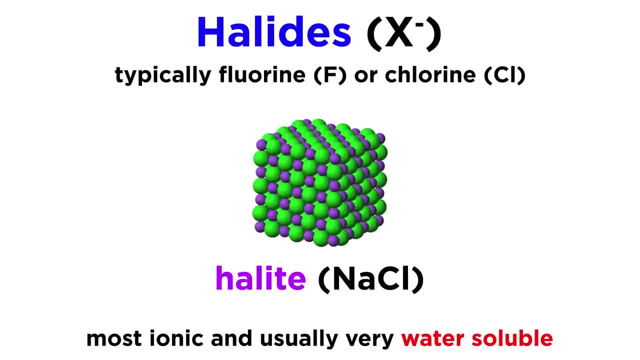 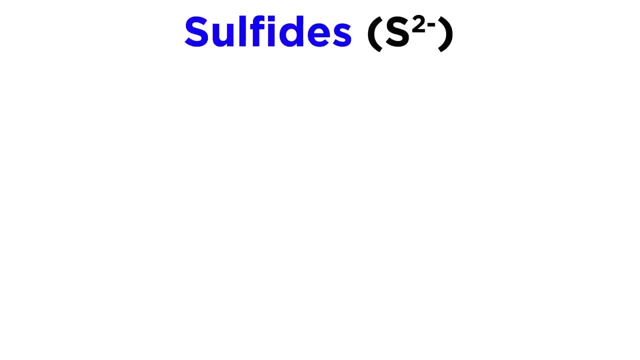 Halite, or sodium chloride, is a common halide mineral, and it often precipitates during the evaporation of seawater. Our final class of minerals that contain a single anion are the sulfides. Unlike the oxides and halides, the bonding in sulfides is very complex and can range. 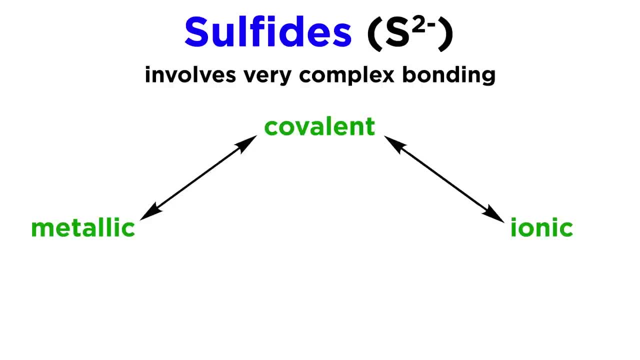 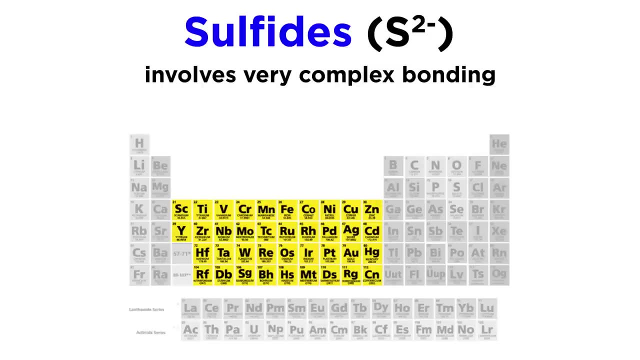 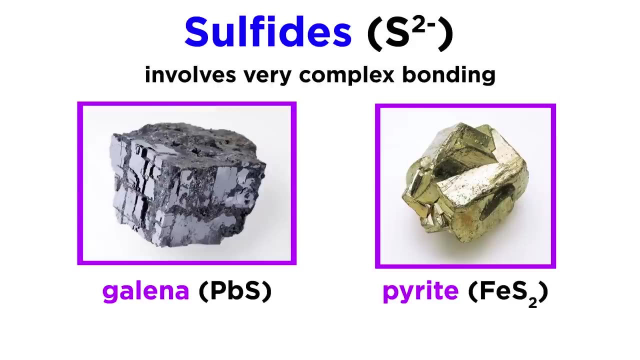 from ionic covalent to metallic covalent, depending on what it is bonding with. Most sulfide minerals are composed of sulfur bonded to a transition metal and often display many of the properties of metals. Incidentally, both galena lead sulfide and pyrite iron disulfide are semiconductors. 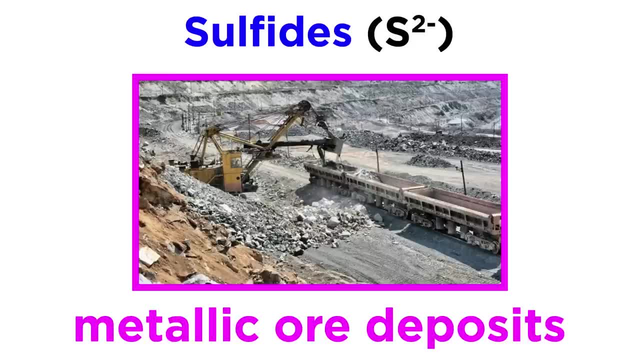 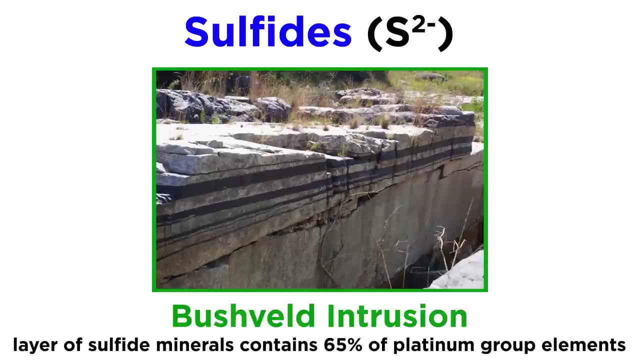 with a metallic luster. Many sulfide minerals are both associated with and hosts of numerous metallic ore deposits. For example, the bush field intrusion, which is a very common mineral, is a very common mineral that is associated with a metallic ore deposit. 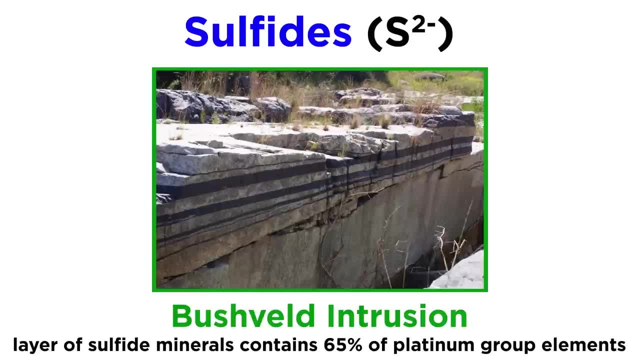 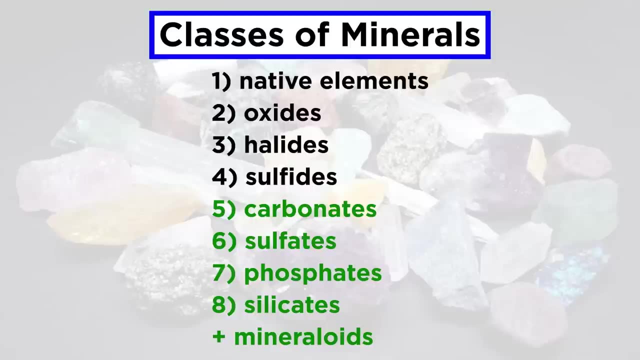 A large intrusion, which is a large intrusive igneous formation in South Africa, possesses a layer of sulfide minerals that contain 65% of the world's reserve of platinum group elements. So that covers four out of the eight classes of minerals. Let's move forward and check out the other half now. 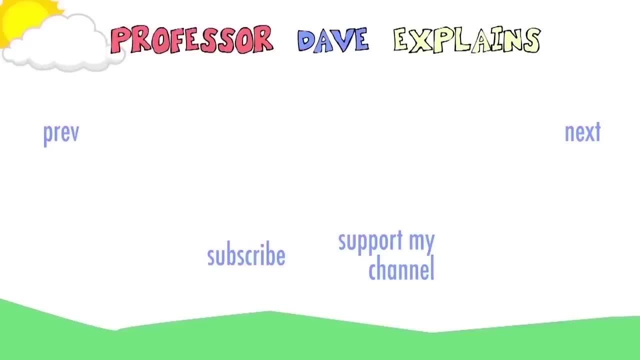 Thanks for watching and I'll see you in the next video. Bye.